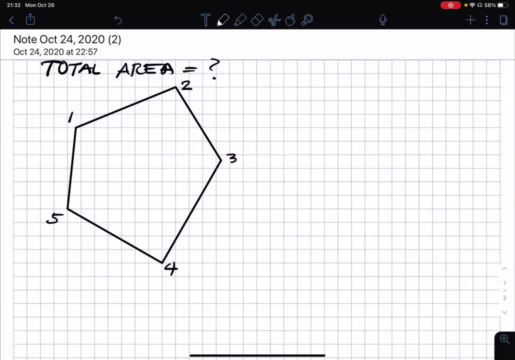 we need a reference point, we need a distance and we also need a reference angle. So in your trigonometry, if you will recall- okay, recall your trigonometry- If you have a triangle and say this is distance A and B and this is your angle alpha. 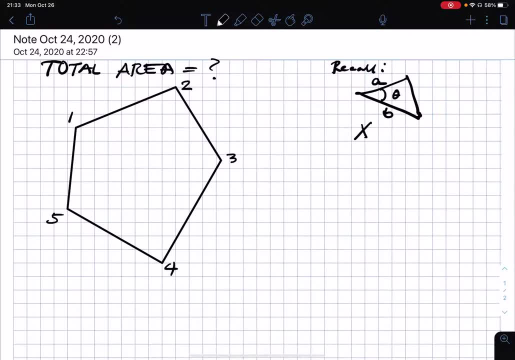 you can calculate the area of a triangle by taking the average of two sides, which is one-half AB, multiplied by sine theta. okay, where theta is your included angle. So this will be our reference formula. Okay, so, in order to apply this one, 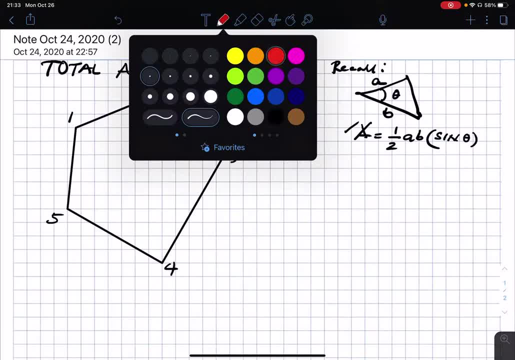 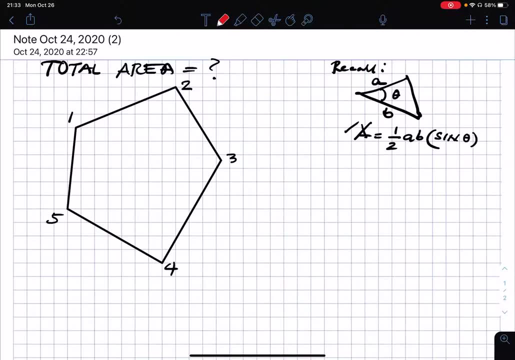 we need a reference point. So in reality, not all points will be accessible. Okay, let's say point one is your most accessible point, So we will use point one as your reference point. So all we need to do is to connect point one to three to form a triangle. that will be your first. 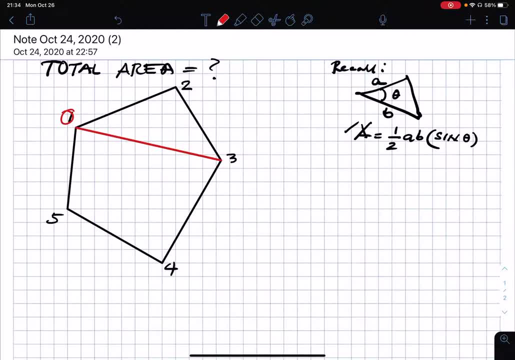 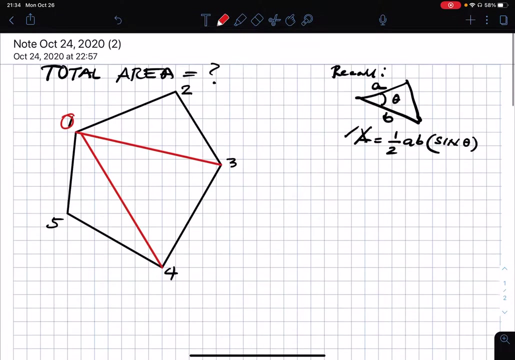 triangle, Then 0.1 to 4 will be your second line. So you have now subdivided a five-sided lots into three triangles. So the next step is to name 1, 2, which is your line, 1, 2, as your, let's say, this is distance x. 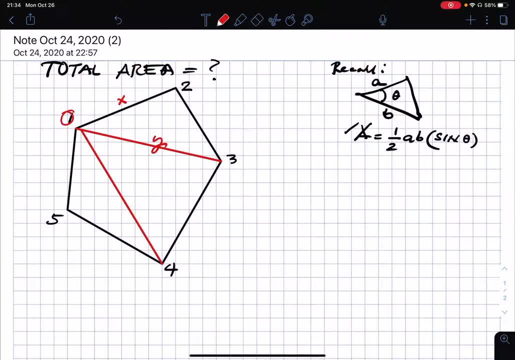 Line 1, 3 as your distance y, And line 1, 4 will be distance z And line 1, 5 will be distance, say, w. So if 1, 0.1 is your reference point, we need the included angle on this side. 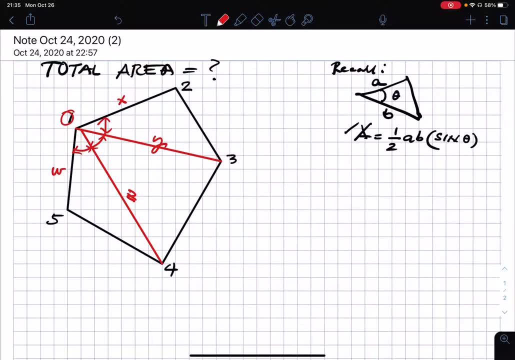 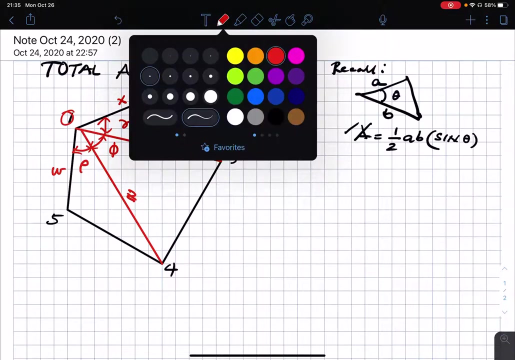 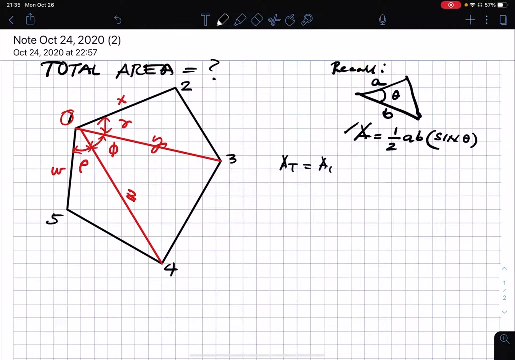 Say, the included angle between x and y is- we call it alpha, Okay. included angle between y and z, we call it angle P And z and w say angle rho. Okay. so by expression we will say that the total area will be area 1 plus area 2 plus area 3.. 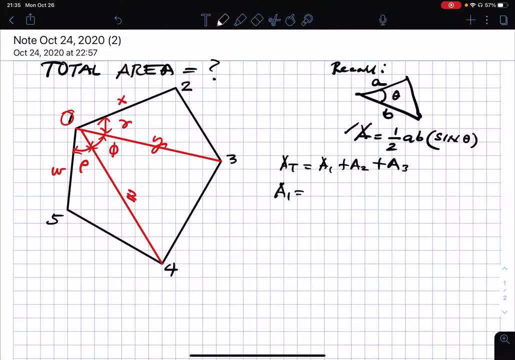 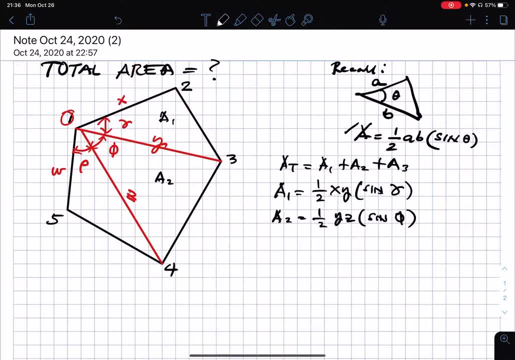 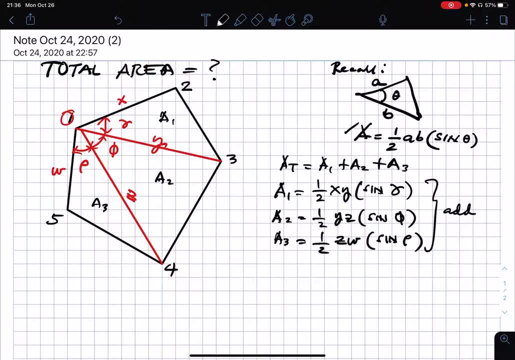 And that will be the total area. Okay, in actual practice again, sometimes line 1,, 2,, 2,, 3,, 3, 4, and 4, 5, the distance might be given, Okay, but the problem is the accessibility. 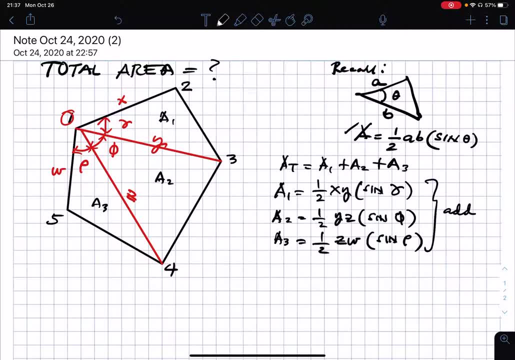 Okay, it's very hard to put a reference point in any of this one, But, following what I did in line in point 1, you can do similar thing in other reference points. All you need to do is two sides and define the angle in between. 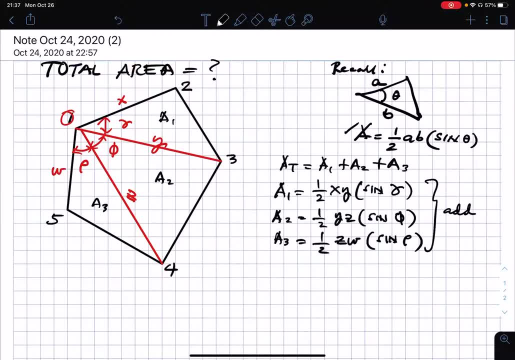 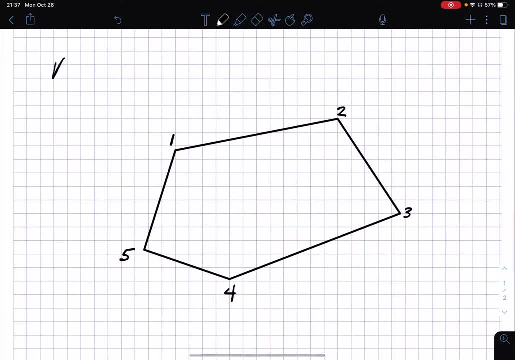 which is what we call the included angle. Okay, let's have another example here. So let's say the total area is unknown And say the given condition is okay, the points around the perimeter is not really accessible. Okay, you cannot stand, or? 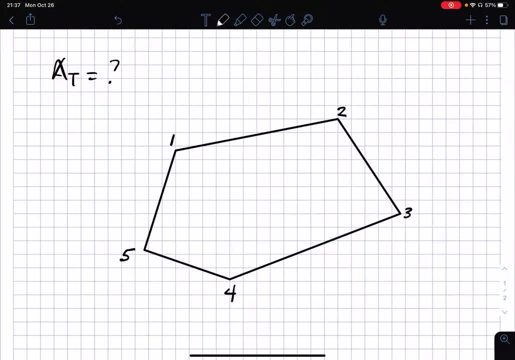 work from that point. But your accessibility is, you can be anywhere on the center. Say okay, that is a center and call it point C. So by using the same principle, all we need to do is to connect the points Say 1 to C. 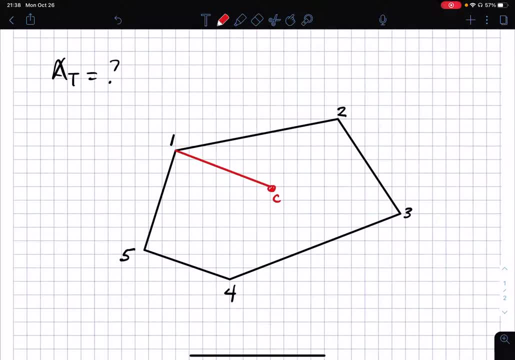 Okay, that's your first point, Then C, Then C to 2, second, then C3,, C4, and C5.. So this will be your area 1,, area 2,, area 3,, area 4,, area 5.. 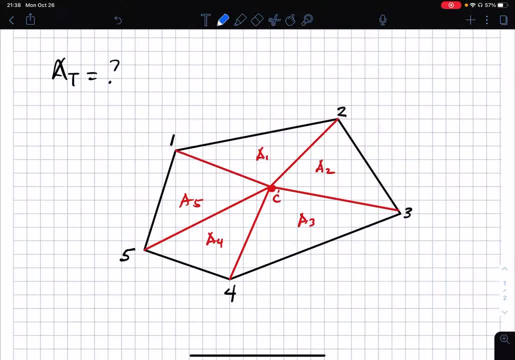 So the next step here is to determine the angle in between. Okay, so say this is alpha, theta, rho, p and tau. So by definition, the area of a triangle is 1 half 2 sides multiplied by the included angle. 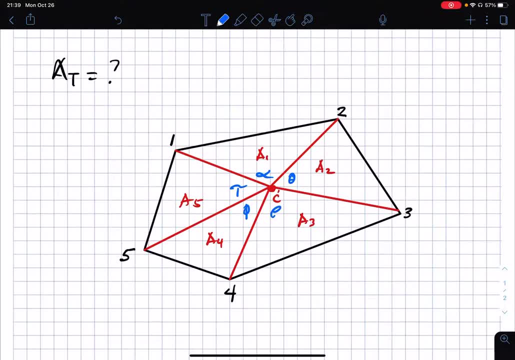 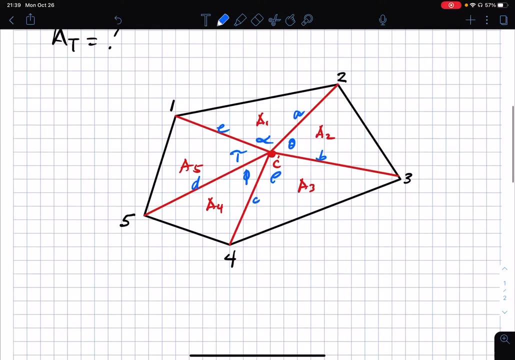 Okay, so we need some distance here. We call this a, so this is a, b, c, d and e. Okay, so area 1, let's use this space here. Okay, area 1.. Okay, Area 2 will now be 1 half a times e multiplied by sine alpha. 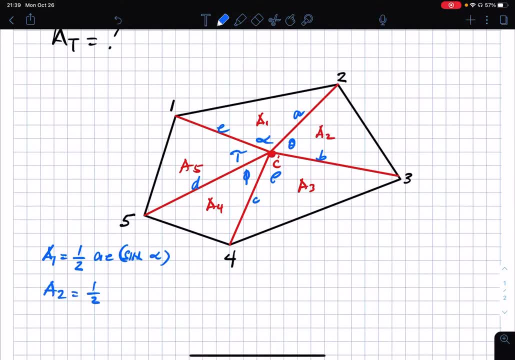 Area 2 is 1 half a times b sine theta. Okay, Okay. Area 3 will be 1 half Okay. Area 4 is 1 half b times c sine rho. Area 4 is 1 half c times d sine p.